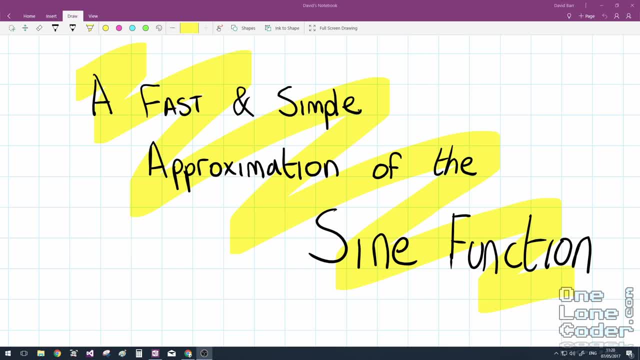 other people use for different platforms. So I'm going to leave all of the caveats and the use cases of this approach to the end of the video and just get stuck in with the guts of it now. Now, if you've watched any of my previous videos on sound synthesis, 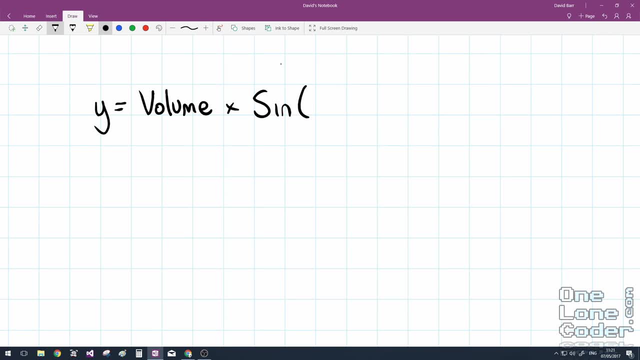 you'll know that we use the sine function a lot and it's usually used in this sort of format where we take the volume times the sine of 2 pi times the frequency of the sound that we want to play times time. And this is great when you have a processing architecture. 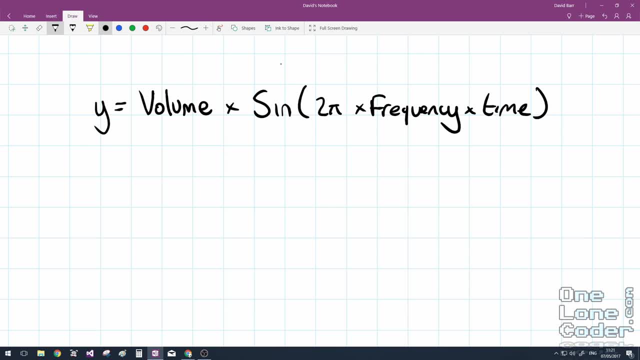 that has the facilities to do these functions. However, my plan is to migrate some of the synthesis code to an embedded systems platform that doesn't have in silicon sine computation. It also has a reasonably low clock function, So I need something that's fast and simple And, because it's audio synthesis, an approximation. 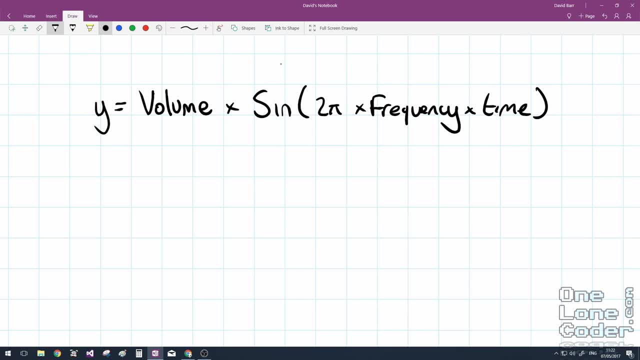 to sine is sufficient. So I'm going to start just by defining the scope of the sine function we're trying to approximate, And the assumptions I'm going to make is that the frequency is always greater than or equal to 0, and the time is always greater than or equal to 0.. 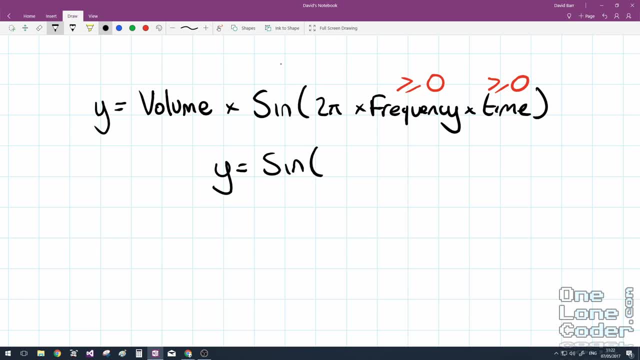 So the final form of our sine function is going to be simply y equals sine of x, where x must be greater than or equal to 0. And, of course, y equals sine of x. Our output is going to be from minus 1 to plus 1.. 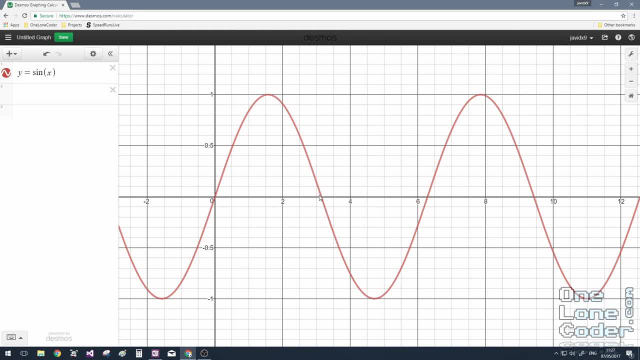 For the uninitiated. this is a sine wave. And here we've got it crossing the axis at pi 2, pi, 3 pi. In fact, it'll do that forever and ever, and ever. And it goes on, and on. 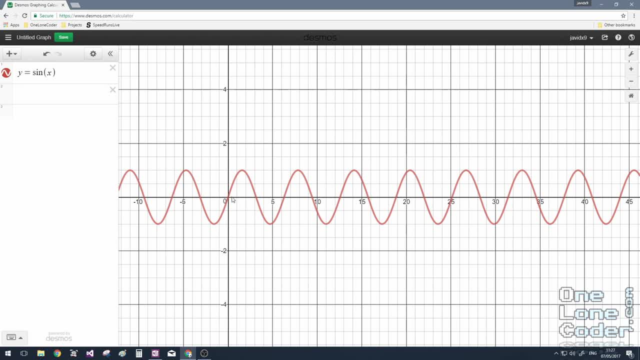 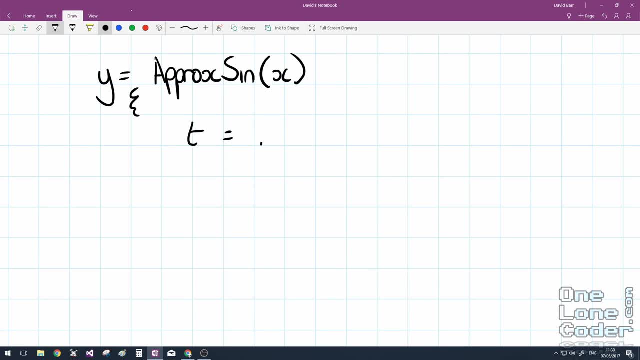 And this is a periodicity, And so our approximation will also need to handle this periodicity, And that can be quite complex. Now, assuming we're using floating point, one way to handle a periodicity would be to use something along the lines of a floating point modulus function, which would take our x input. 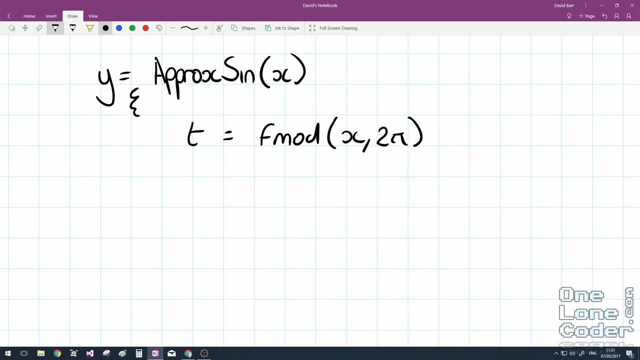 and we could modulate that by 2 pi, which of course means for every value over 2 pi it wraps around to 0. So we can use basically the remainder as the index into our approximation function later on. However, this function is complex, requiring a floating point divide, And it may not be. 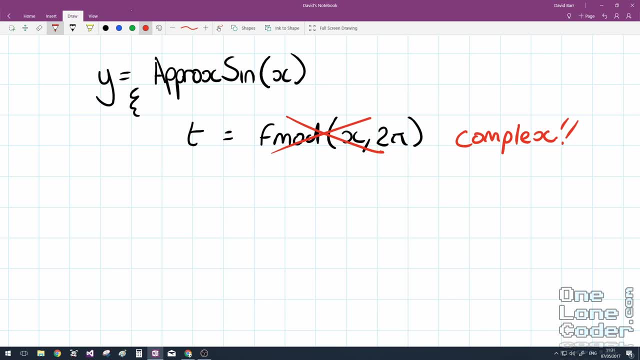 supported on all platforms, And I think there's a better way to do this, And what I'm going to do instead is normalize the input to between 0 and 1.. Of course, I'm going to do that by dividing it by 2 pi. In this case. I want to keep it no divides, because 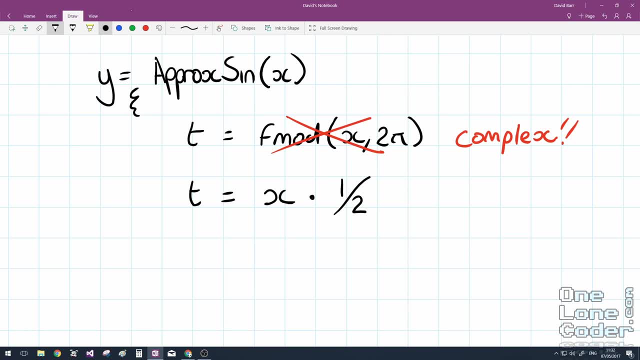 they're usually quite complicated to do, So I'm going to multiply it by a constant 1 over 2 pi. So this means now 2 pi is equal to 1, and 0 is equal to 0, and pi is equal to half. 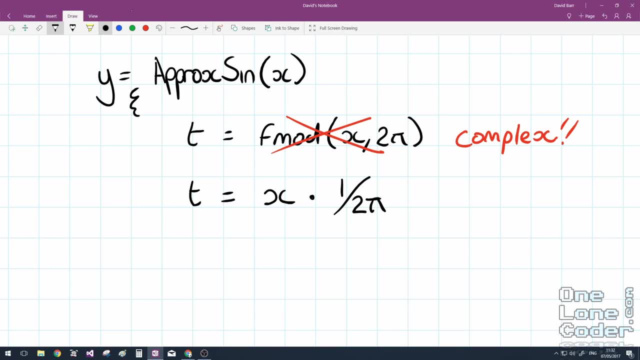 And instead of requiring us to do some arbitrary modulus to some complex number like this, instead we can simply hack using a floating point to integer conversion So we can take our normalized value and subtract from it the integer value instead. So this will always give us a remainder between 0 and 1.. And just in case your language doesn't: 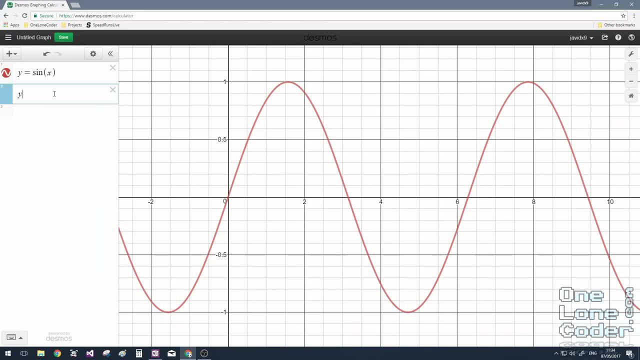 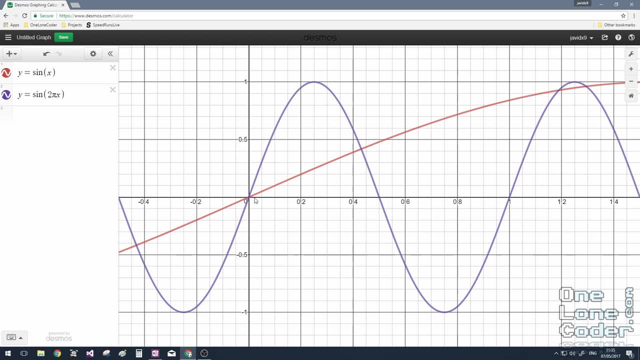 support this. it's the equivalent of using, say, the floor function. If I graph what this looks like, we'll see. it remains a sine function, but it looks like a high frequency And here- I've just zoomed in on it- We can see the original sine wave in the background. and the new y equals sine 2 pi x here where the input is 0.. And now we can see that we've got the original sine wave in the background and the new y equals sine 2 pi x here where the input is 0.. So we can take our normalized value and subtract from it the integer value instead. So instead of having anySure demarcation, 9 local capital letters of the number terms, we have up to 6 couples in here Once we've reach 0, we have our diagonal learning and now we can calculate vec2.. 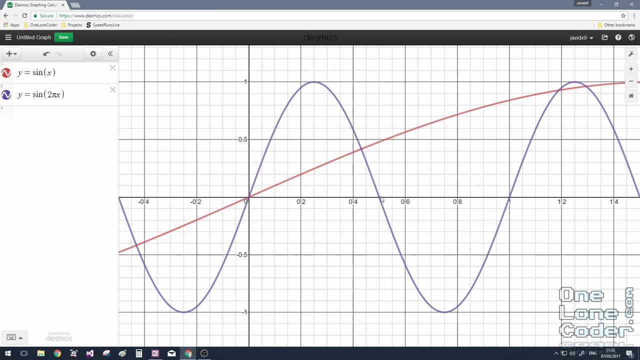 So whatever we want to show into vec2, we are going to just split byalnız 결 немнож and we'll take 2.. This is cost to sine���ales, And we'll do theurun PhD from y equals sine asriθHyperl Nousso to it will be. 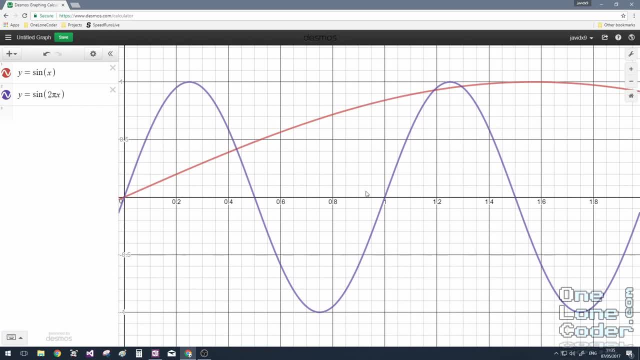 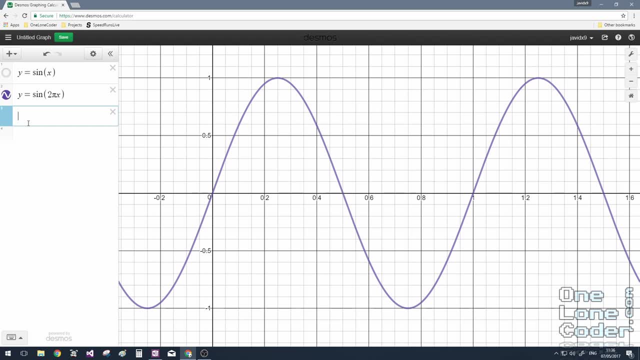 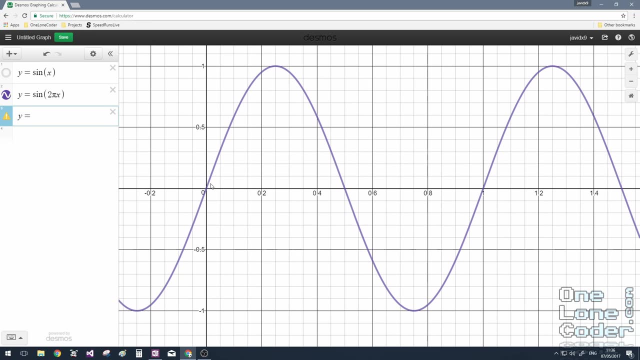 And so forth along. So now we've got this easy way of calculating the remainder without using the floating point modulus. I'm going to show two approximations, but I'm going to start off with a quadratic approximation to sine Queue. To calculate this, I know that my roots for at least one of the parabolas is 0 and 0.5,. 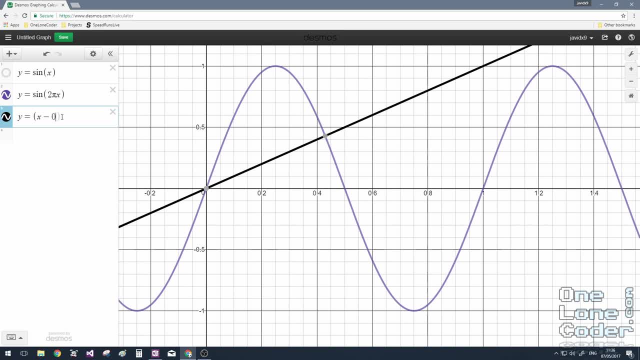 So let's just start with a very basic quadratic calculation with a root at 0 and a root at 0.5.. First thing I can see is it's upside down, so I'll throw a minus sign in there just to invert it the right way up and so we can see it crosses now at the same places, but it needs. 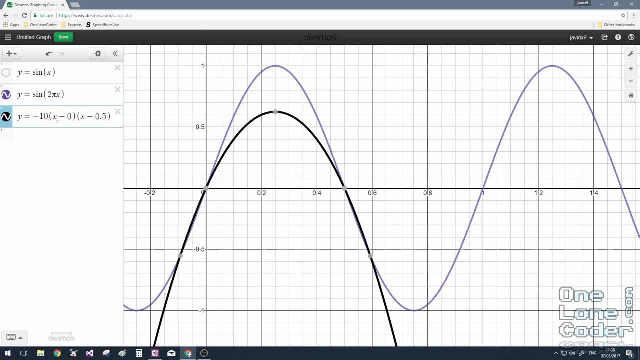 some scaling. I'm just going to take a guess at the scaling and we'll say it's 10, oh, it's not quite enough, so let's try 20, looks a bit too much. let's try somewhere in the middle. 15,, no 16, oh, 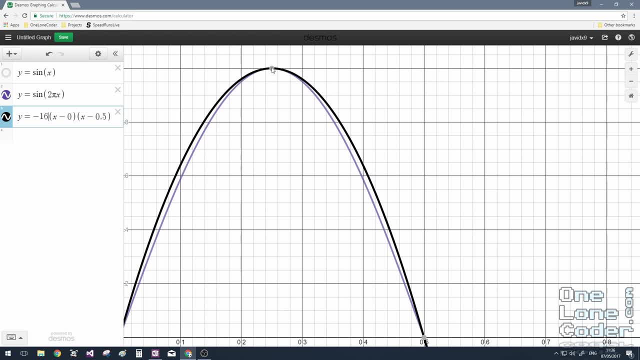 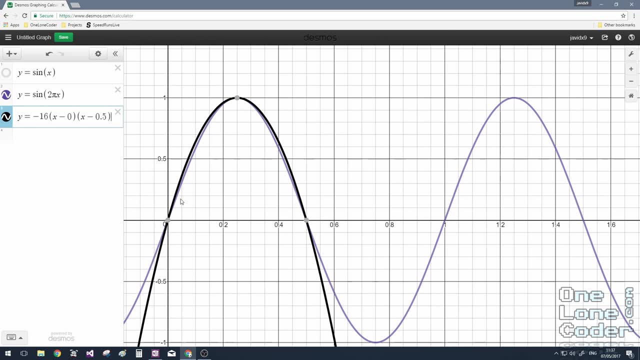 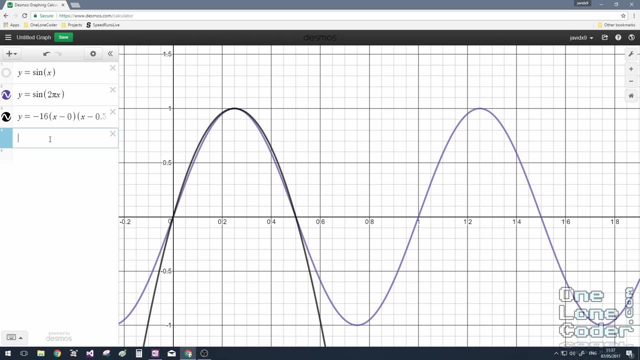 that one looks good. so let's just quickly zoom in and we see it's absolutely perfect. so it gives us a value up to a maximum of 1.. That's handled the positive side of the sine wave. Let's now look at a quadratic equation for the negative side. 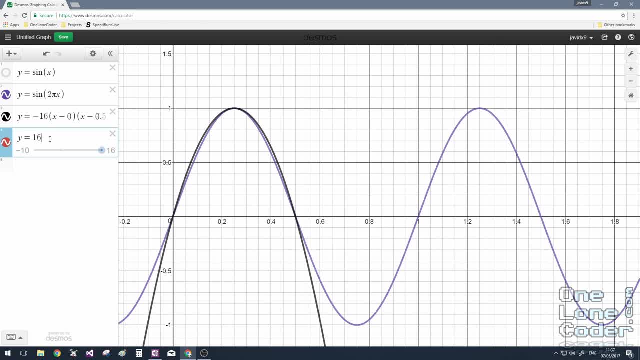 So we know that we've got a scaling factor already and we know that we don't need it to be minus 16 this time. probably 16 will do, because it's the parabola that's the right way up. But our roots have changed. 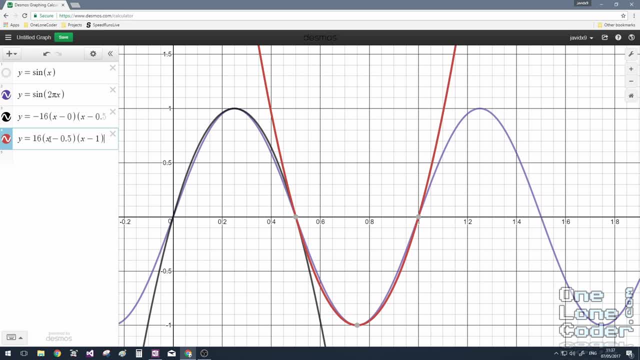 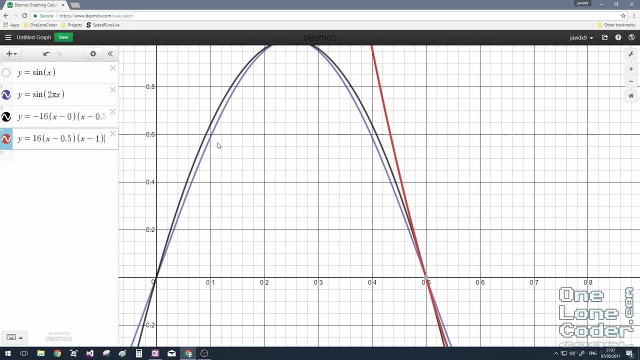 So now it's a minus 16. 0.5 and 1.. So using two parabolas we can roughly approximate the sine wave and we can see it is an approximation. it doesn't perfectly follow the purple sine wave in the background, but you know what it's. 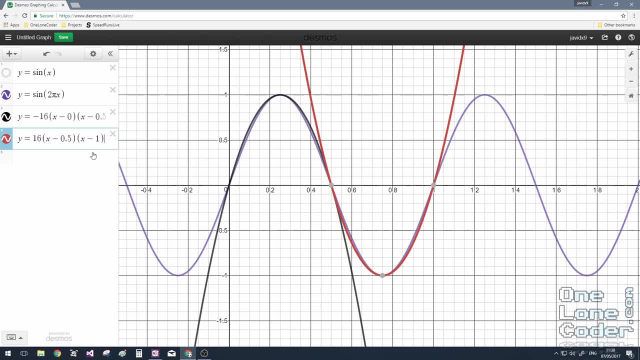 probably good enough for audio synthesis. and we can decide which equation to use, based on the input value of x: if it's greater than 0.5, we use our positive parabola, and if it's less than 0.5, we use our negative parabola. 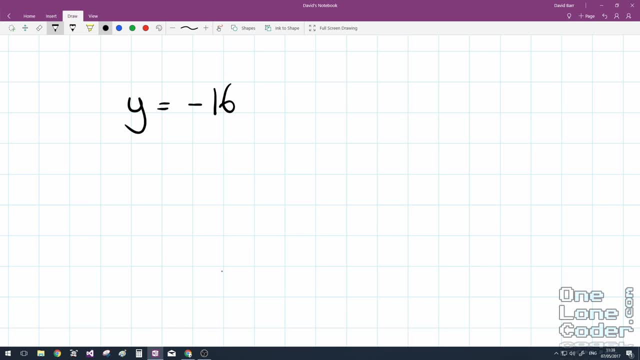 Let's just have a look at the numbers here. so if we just copy over our first half, which was minus 16, x take 0 and x take 0.5 roots, and if we just tidy this up a little bit, we've got minus 16 x squared. take 0 x, take 0.5 x and the constant disappears 0 times. 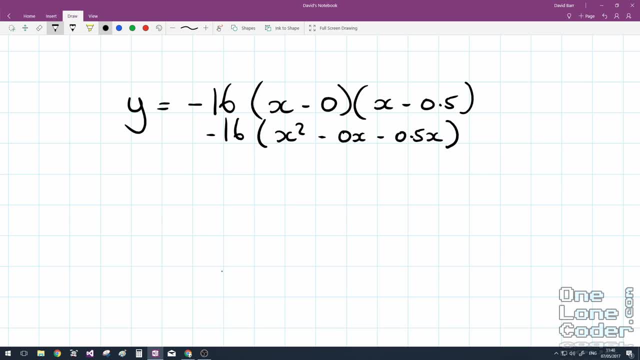 0.5, that goes away and we fill that out now to be 16 minus 16 x squared. take 8 x And programmers get very excited when they see 16s and 8s and 4s and 2s, because it usually 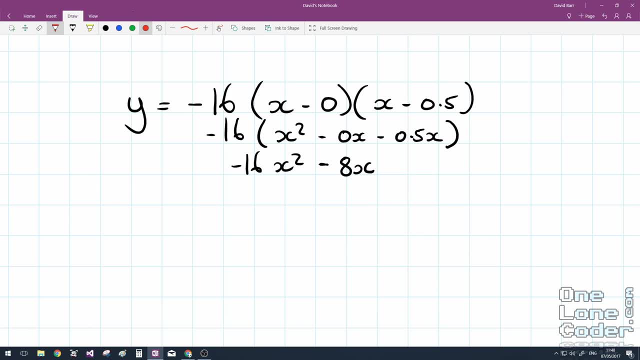 means there's some scope for some bit field manipulation to more optimise the mathematics involved. Now we're doing this all in floating point, but if I did want to convert this to a fixed point, of course, multiplying by 16 is the equivalent of shifting 4 bits and multiplying by 8 is. 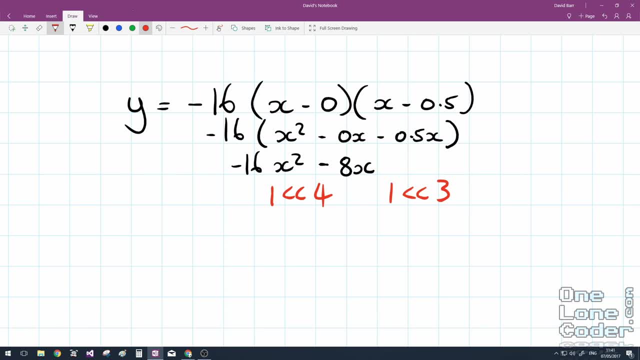 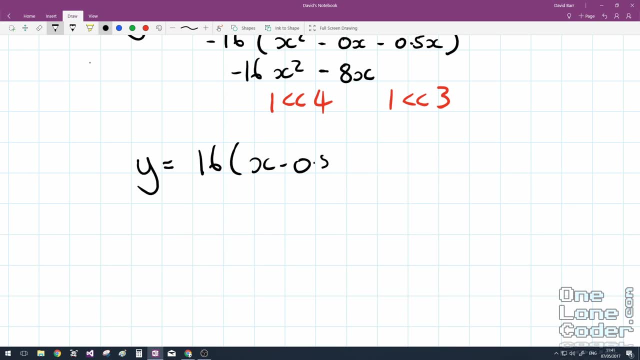 the equivalent of shifting by 3 bits. So there's potential for optimisation here. Let's also consider the other half of our parabola, which was 16: x take 0.5, x squared 0.5 and x take 1, and if we expand this out again, we've now got x squared take 0.5, x take. 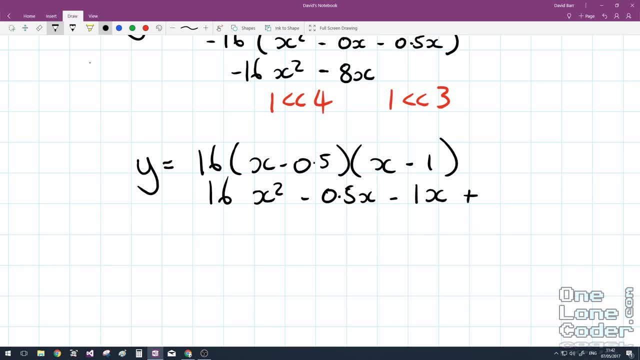 1 x plus half. Now I'm not going to group up the 0.5 and the 1 for exactly the same reasons as labelled above, because if we draw this out now by multiplying everything by 16, we get our 16 x squared. take: 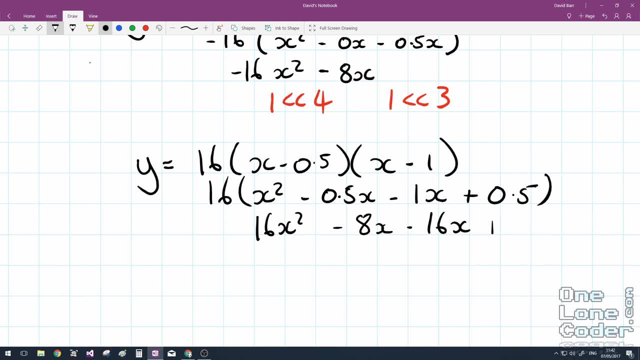 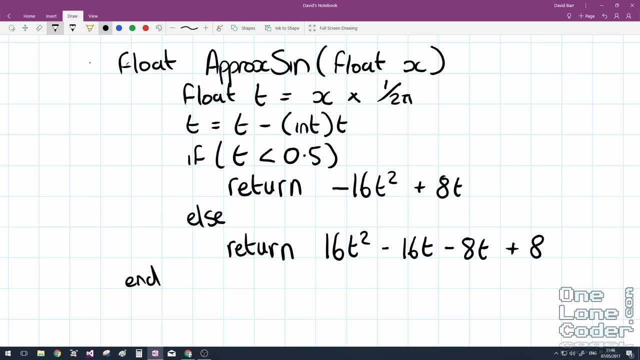 8 x. take 16 x plus 8.. And again we remain with coefficients here which are multiples of 2. Here I've drawn out the pseudocode for our approximate sine function. I'm going to assume that we're using 32 bit floats for all of this. and here we can see: 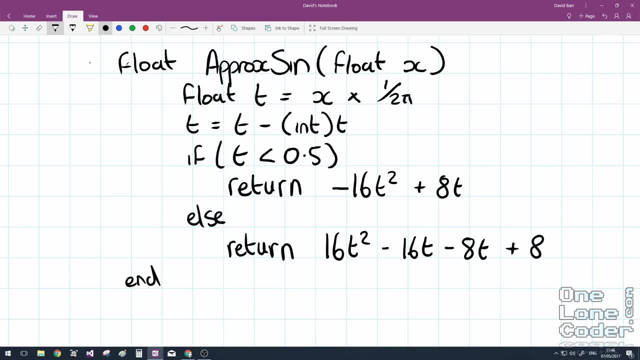 that I first of all scale the input to normalise it between 0 and 1.. I then do this nice way of doing a modulus just by taking the integer proportion away from the input. It's just, then, a question of making a decision between which parabola you use, whether we 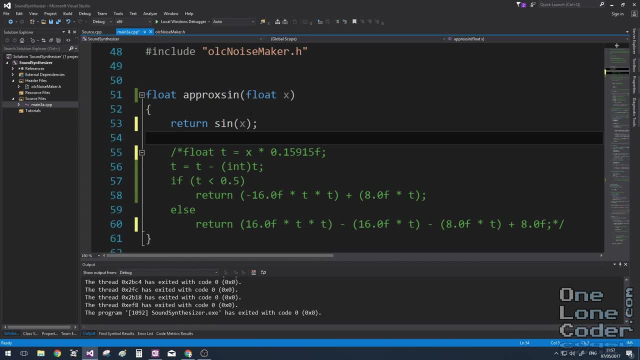 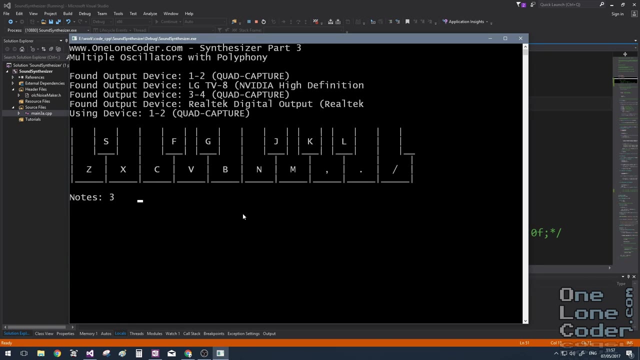 want the first half or the second half. So here I've overridden the sine function in my synthesiser with the approximate sine function you've just seen me type out and I'm just going to play it and we'll have a listen. So this is just a pure sine wave. so this is what a sine wave sounds like in this system. 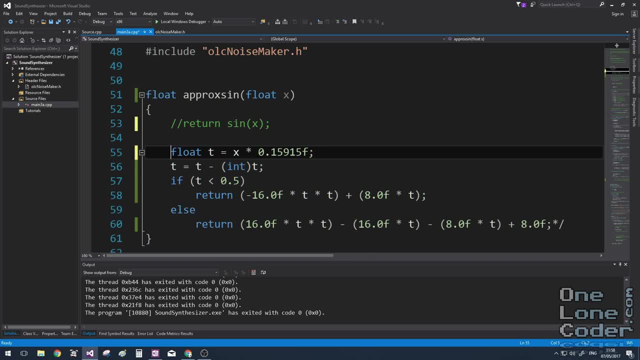 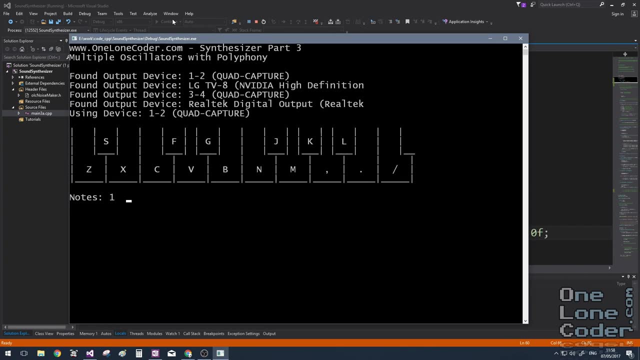 And now if I remove the sine and replace it with our approximation, You can hear it's not a bad sine wave. it does actually sound like a little bit of a square wave and if we look at the graphs we can see why. Our approximation, the black: 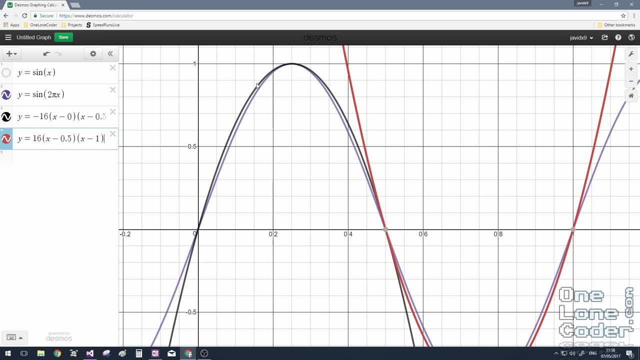 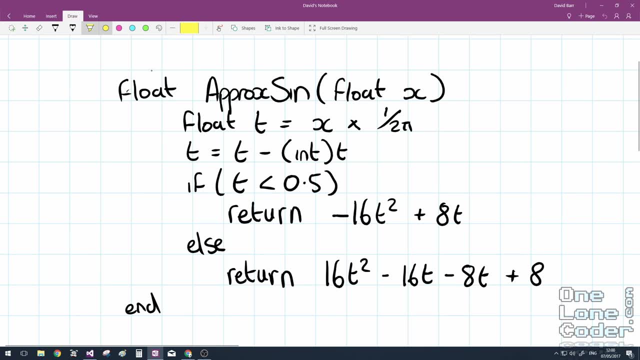 line is always larger than the actual sine wave itself. it bulges out, so it's approaching a square wave very slightly. That said, I think it's quite a good approximation. Now I'm sure there'll be some programmers out there that really don't like having a branch. 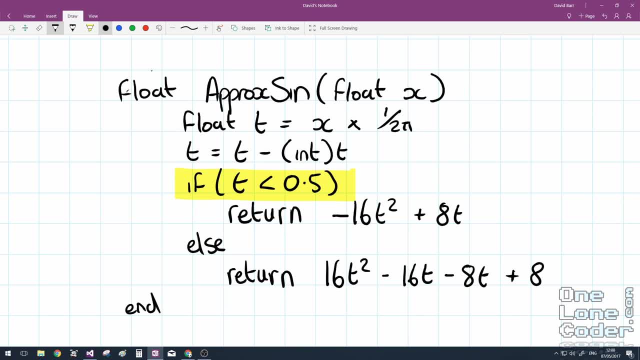 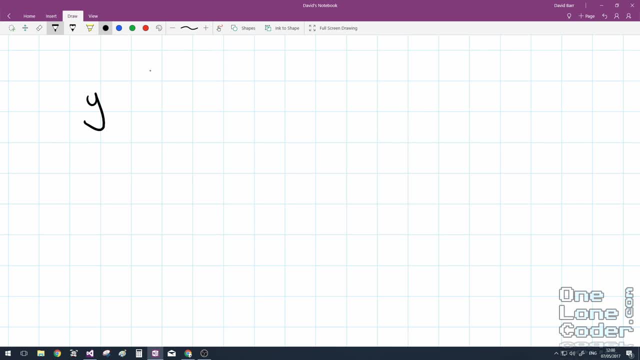 condition in the middle of the continuous function approximation. One way to do this would be to use an approximation that has three roots instead, so a cubic, and I suppose it would look something like this: so we would have y equals x minus 0, because we know that's. 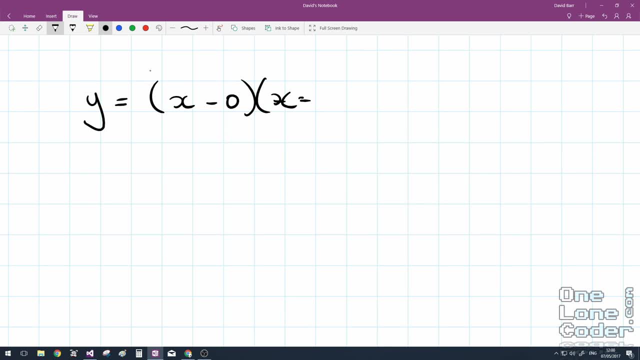 one of our roots we know. the next root is x minus 0.5, which would be equivalent to pi in our normalised space and x minus 1.. Let's take this over to the graphing platform and have a look. 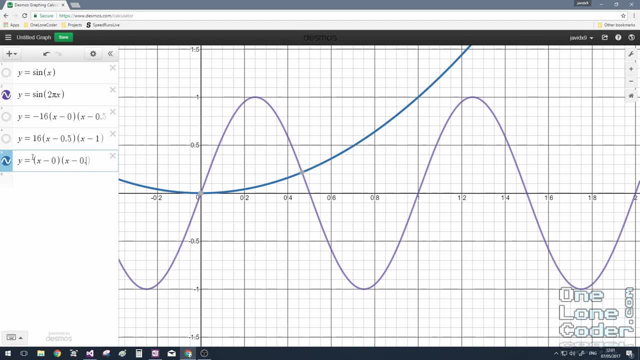 So our first root is at 0,, our second root is at 0.5, and our third root is at 1.. And we can see that the roots are fine. but again we've got a scaling issue, so let's just have. 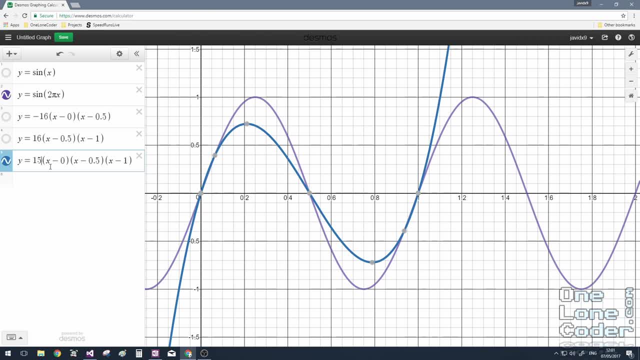 a quick guess. I'm sure there's some maths purists out there that might be able to work this out. 15 is not quite enough, 20 is not quite enough, 21 is a bit too much. so somewhere between there, In fact, I know, it turns out that 785 actually gives us a presumptuous. 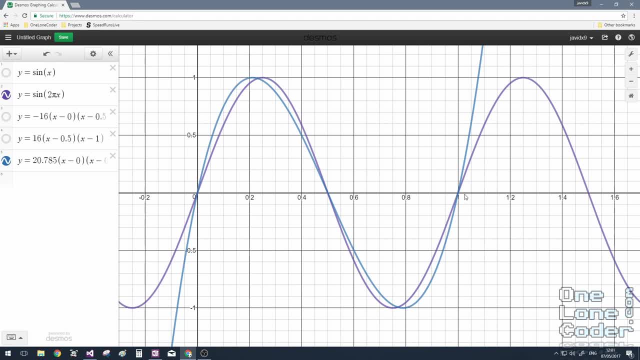 value. but if we do the same thing here, then we can get the same value. we can get a pretty precise 1 for the output Now, using exactly the same periodicity calculator that we used for the quadratic. we can use the same for the cubic and we can see that this time the peak happens before the sine. 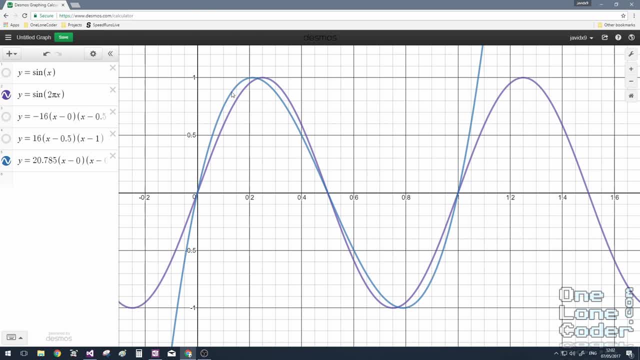 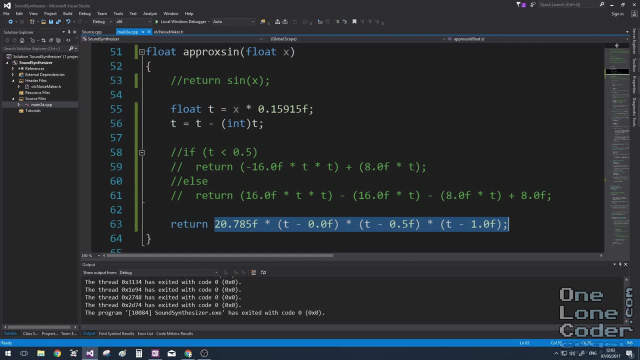 wave, and the peak happens after the sine wave, and so, by definition, this approximation is not so much a sine wave, but it's a very slight sawtooth wave, and so we must listen to it. So here, in exactly the same function, you can see, I've just typed in the code, exactly. 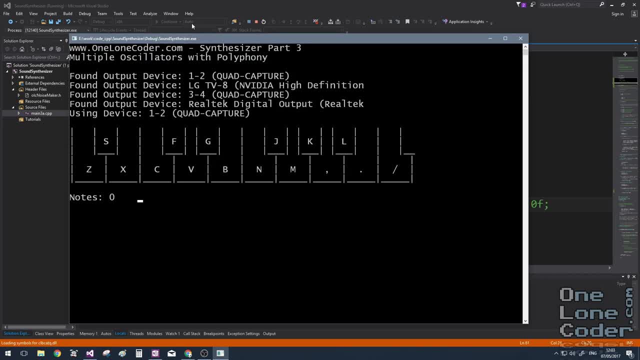 I've not tried to reduce it to look at any interesting coefficients that we might be. have a listen Now. that sounds absolutely lovely. there's just something really nice about that tone. If it sounds a little bit garbled, that will be down to the YouTube audio compression. 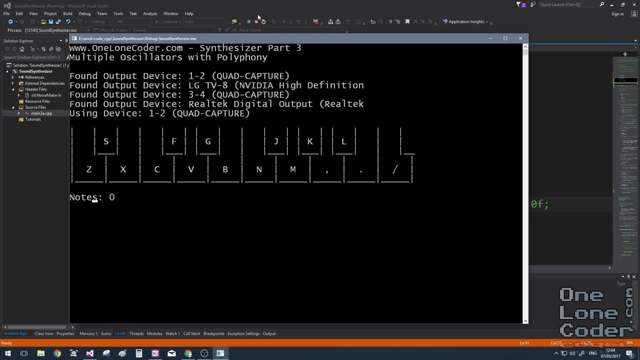 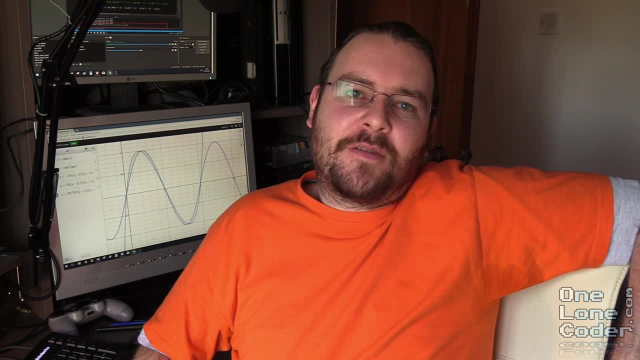 So I recommend that you get the code from GitHub, follow the link below and try it out for yourself. At the start of this video I mentioned that there are always caveats when approximating other functions. For really large values of x, the floating point precision would start to work. 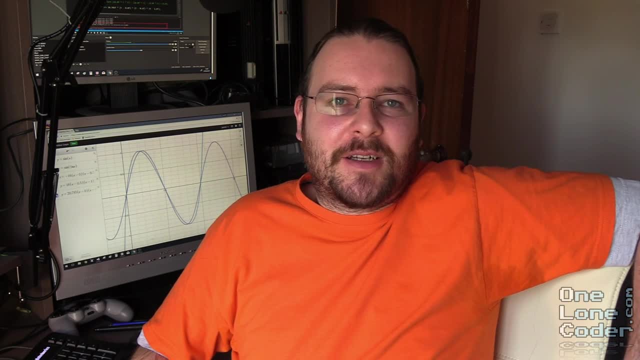 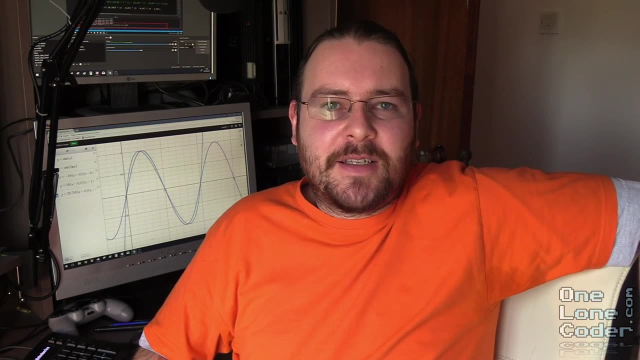 against you, which may produce some very interesting audio artifacts. perhaps a gradual degradation of the audio quality over time. It might sound really cool, but it's always worth thinking about the use cases for your approximation. On a modern desktop computer you're probably better. 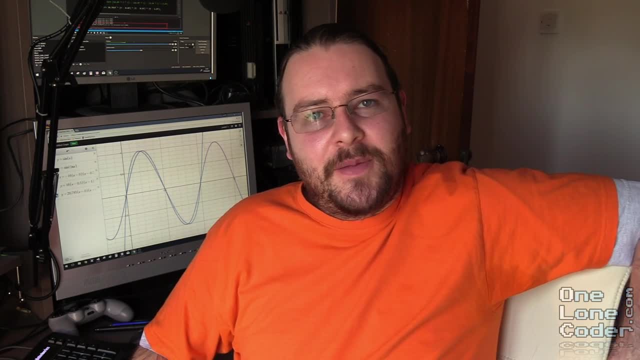 off just using the sign directly. There'll be dedicated silicon on the CPU for processing sign and cos and tan and all the others. Popular methods in times gone by were to use lookup tables. that did the approximation for you. However, on modern architectures these are probably more likely just